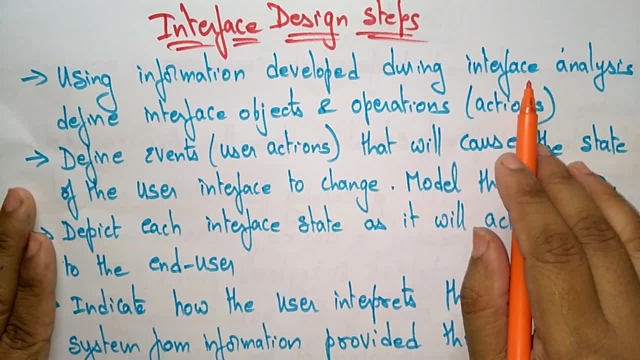 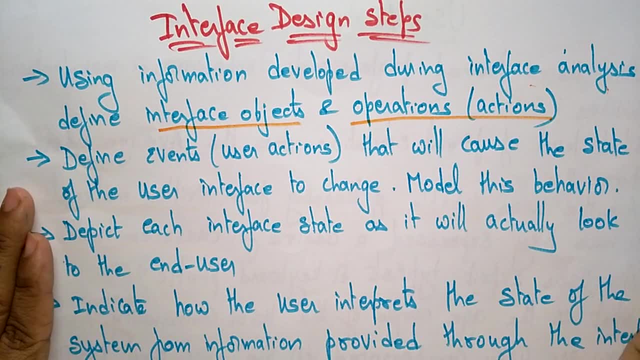 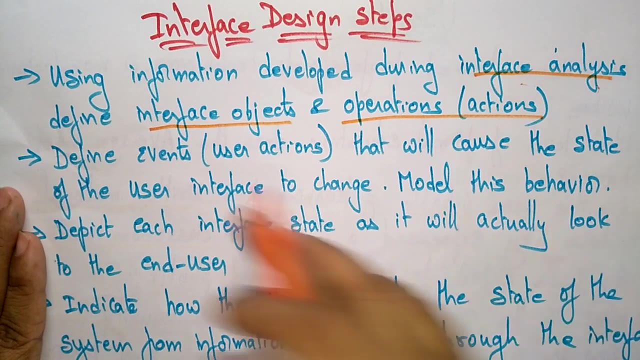 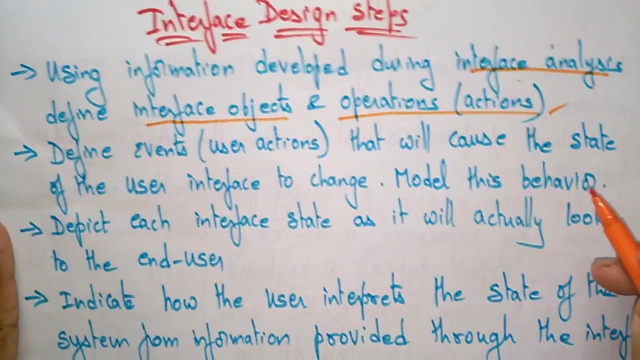 First, using information developed during interface analysis, you have to define interface objects and operations. So, by using the information of developed during interface analysis, we will gather some information. Okay, with the help of that information, we have to define what are the objects- interface objects- and what are the operations that we have to be performed. So that is the first step. Next, define events. 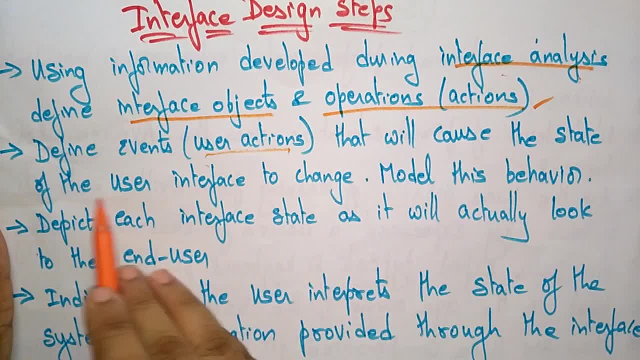 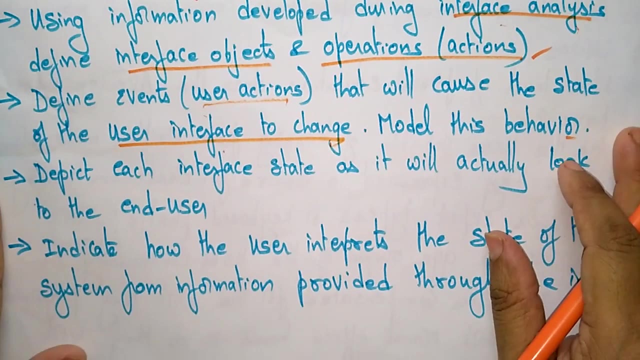 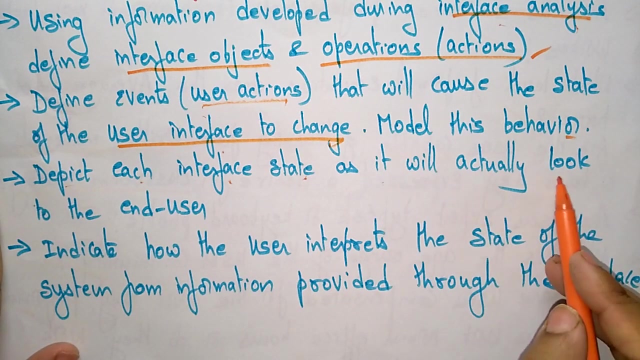 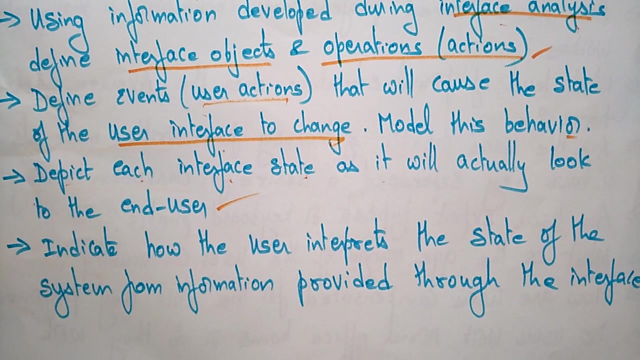 Means, that is, the user actions that will cause this State of the user interface to change. Model this behavior Means, you have to think, identify. is there any event that cause the state of the user interface is going to be changed? That you have to be identified. Next, depict each interface state. So you have to depict each interface state as it will actually look to the end user. So you have to create like that. You have to depict each interface state, whatever the states that will be present in each interface state. 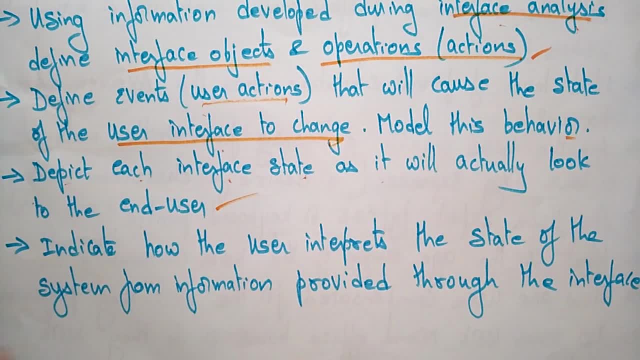 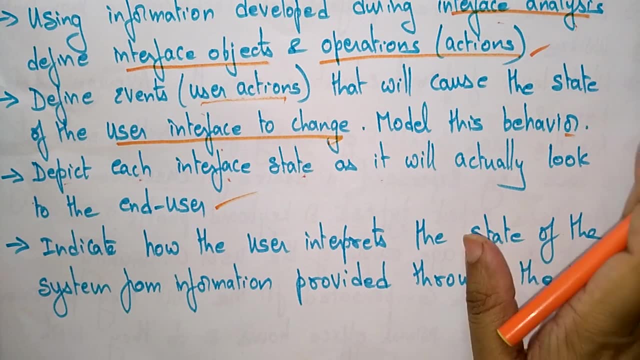 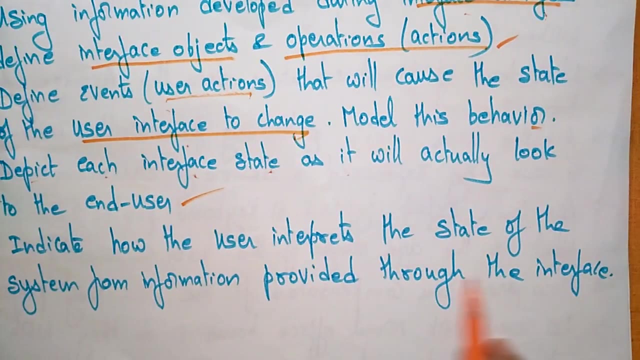 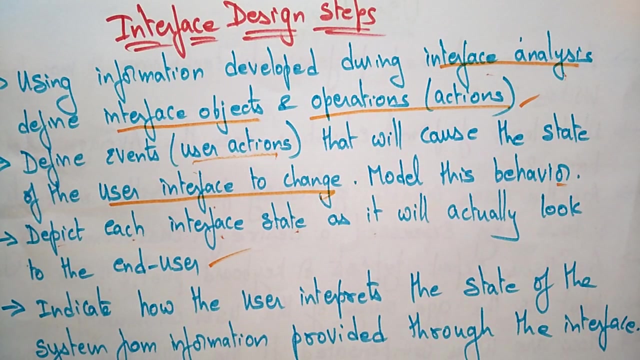 Interface, whether it is analysis phase, user phase, web phase, anything. So in each interface state, as it will actually look to the end user or not, we have to be checked, Indicate how the user interprets the state of the system from information provided through the interface. So these are the design interface design steps that we have to be followed for designing the interface. Okay, now let us see the interface design patterns. 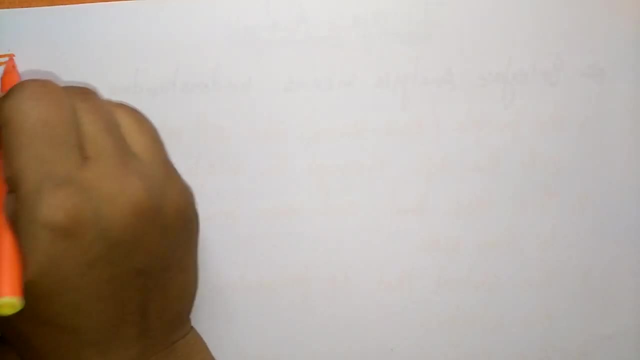 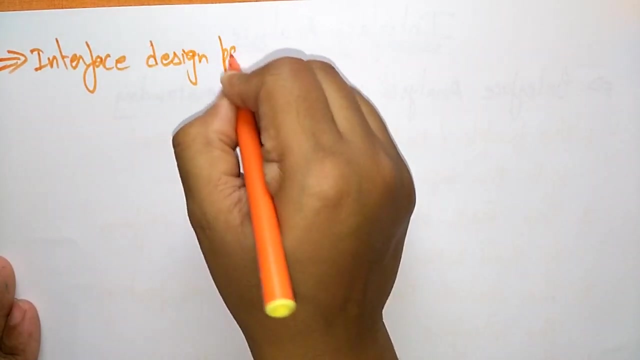 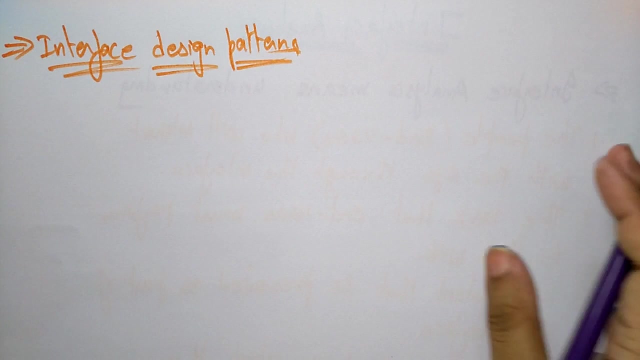 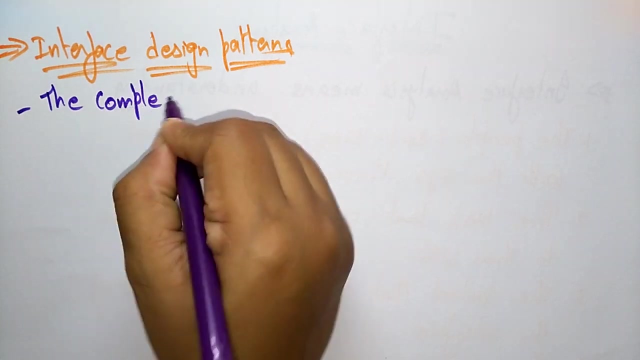 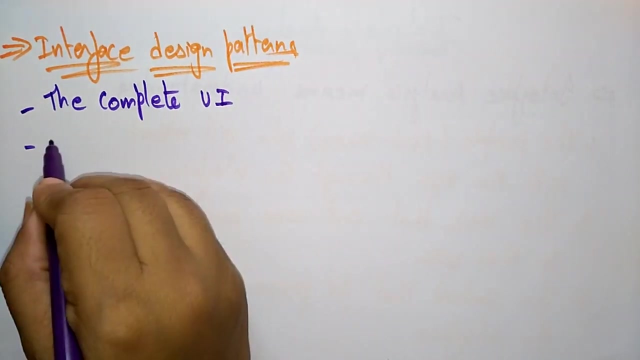 So what are the interface design patterns? So what are the different patterns that will be provided for interface design? The patterns are available for the complete user interface. The patterns are available for complete user interface interface and the patterns will be available for page layouts, for designing the page layouts. 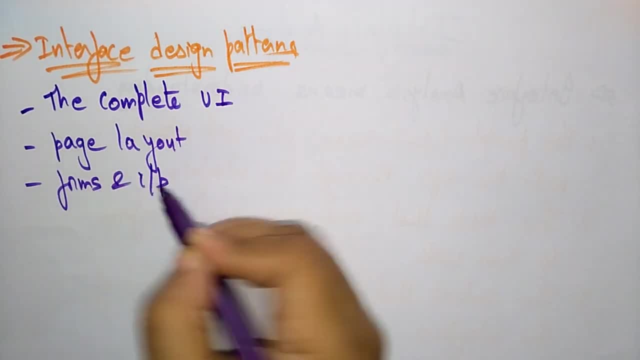 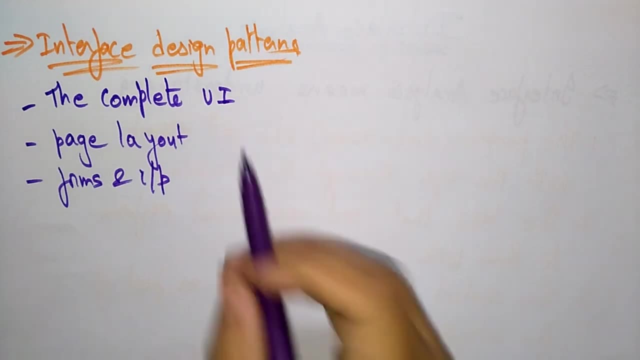 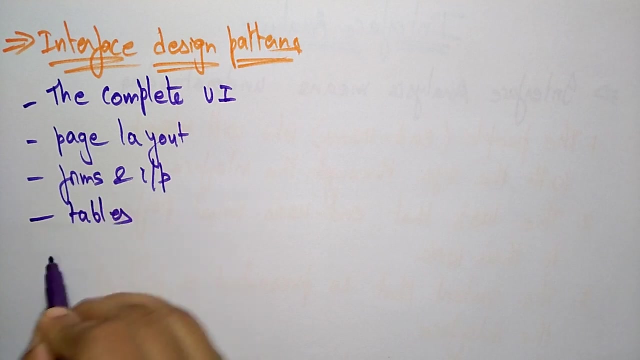 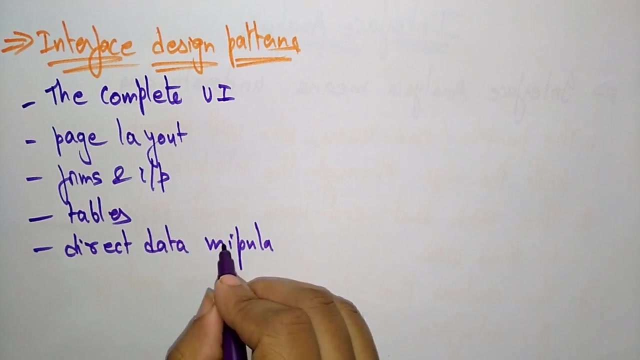 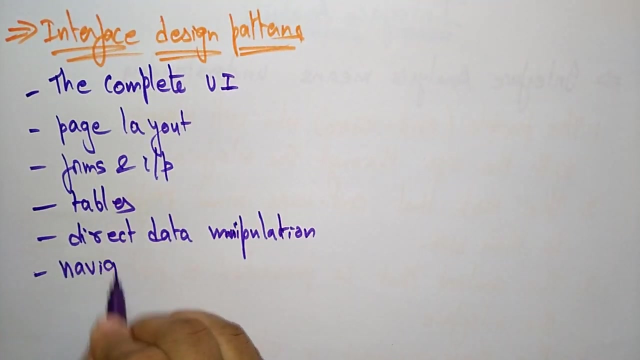 and for forms and inputs. so for forms and inputs, there are different patterns are available. okay, to interface the design patterns. so there are different patterns are available. the complete user interface will be provided for you, or simply you can provide, you can provide a means. It's a page layout. Templates will be provided for you, Already built forms and inputs will be provided. Tables, Direct data manipulations- Sorry, Manipulations- Navigation. So navigation is already implemented. 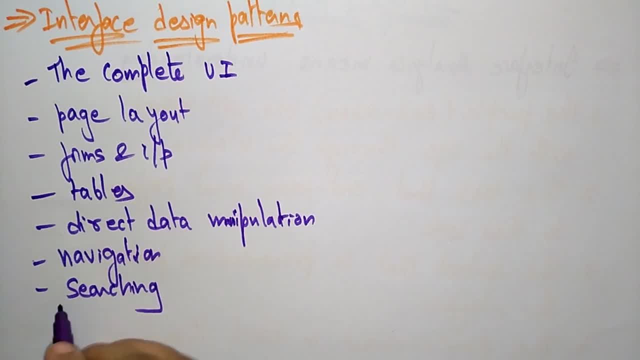 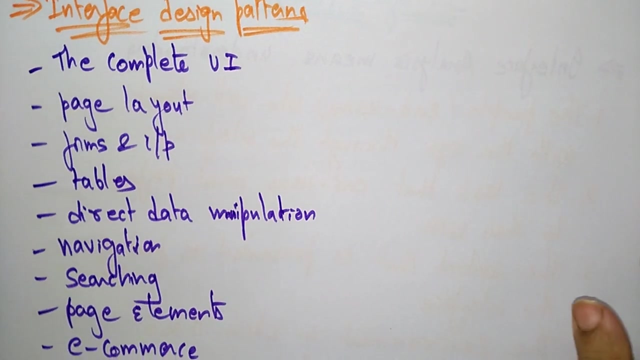 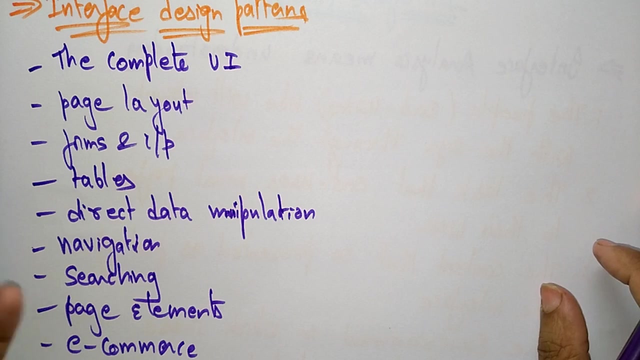 Searching. The searching code is already there, Page elements, Page elements and e-commerce. So these are all the different patterns that are available for interface, the design. Okay, Whatever, it is a user interface. So if you want to design a user interface, that should already the patterns are available, The different patterns that are available for the complete user interface: Page layout, Forms and inputs, Tables, Direct data manipulations. 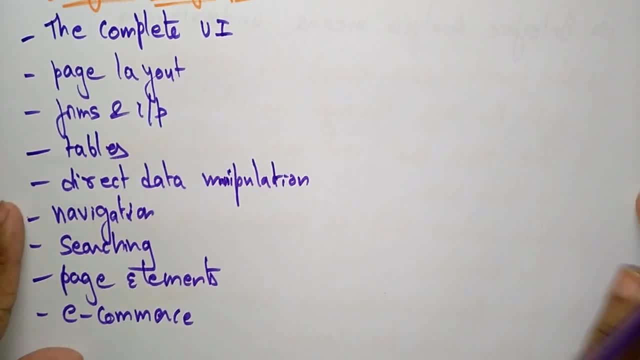 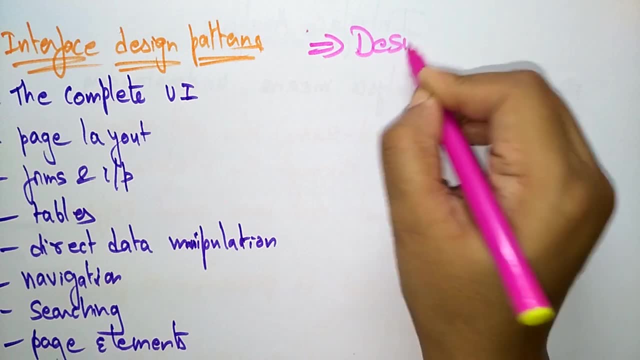 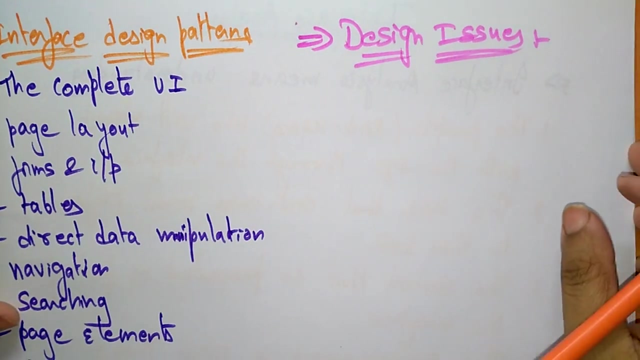 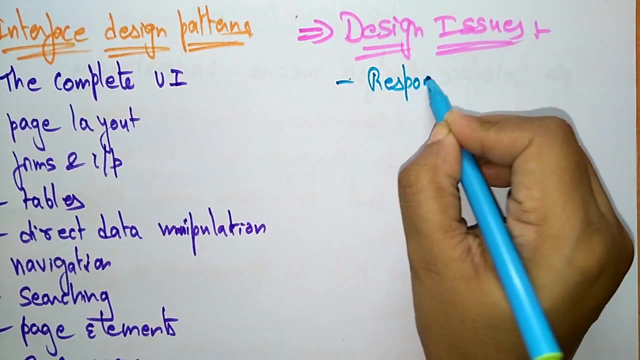 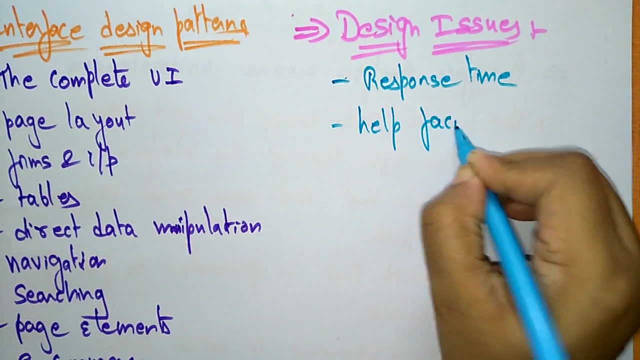 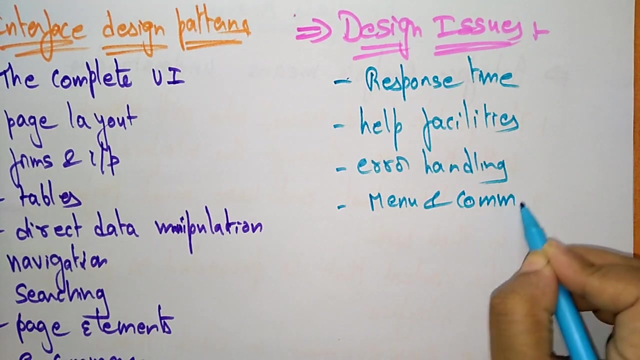 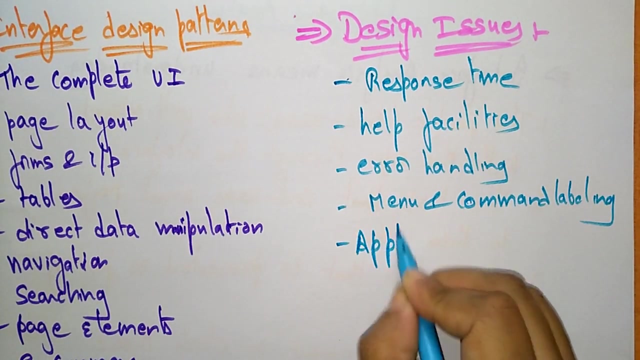 Navigation, Searching Page elements and e-commerce. Now let us discuss about the design issues. that will Design issues. So what are the design issues in this analysis and the design? The design issues are: Response time, Help facilities, Help facilities, Error handling, Error handling, Menu and command labeling. Menu and command labeling, Application accessibility. Application accessibility And internationalization. 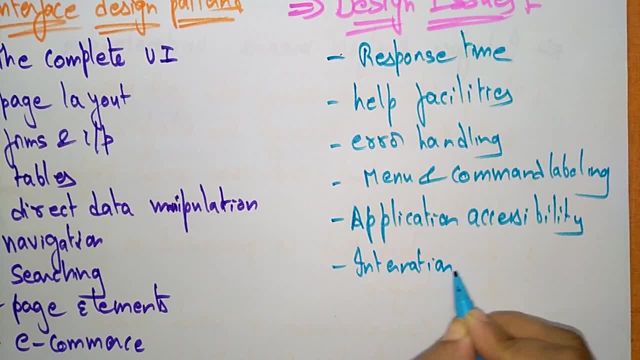 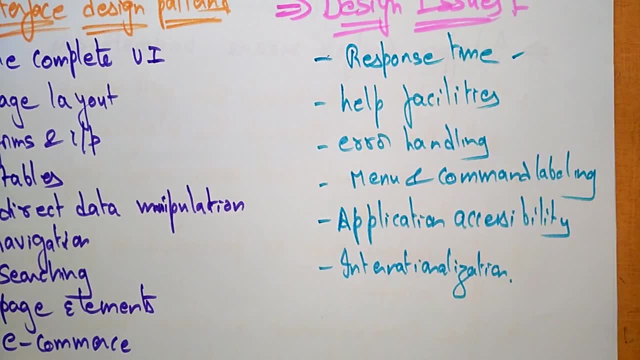 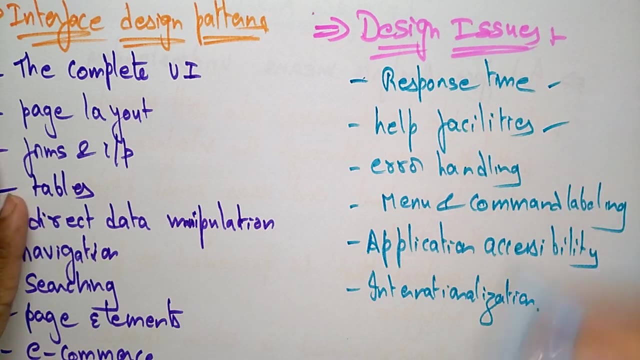 meaningful education. So these are the different design issues that may problems that may occur in the. In the case of response time, Whether the interface that is respond, how much time it takes to respond, Help facilities are provided or not. Is there an error handling technique? will be there or not? 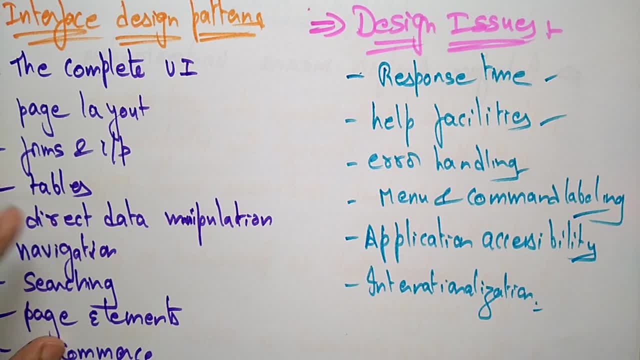 Manual on LI piano Application, accessibility and internationalization. So these are all some design issues for analyzing and design. I want to say thank you to students, staff and the staff for lights. What a plastic box appeared next to it. Is that a very old book?